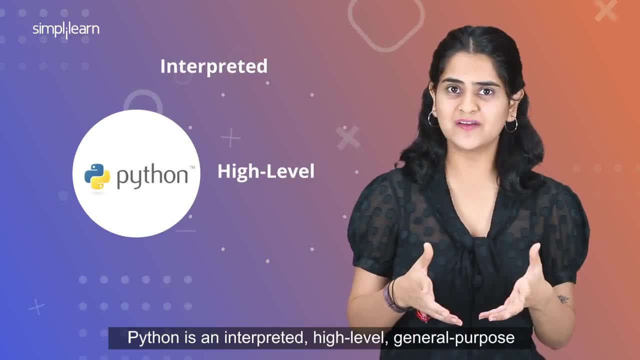 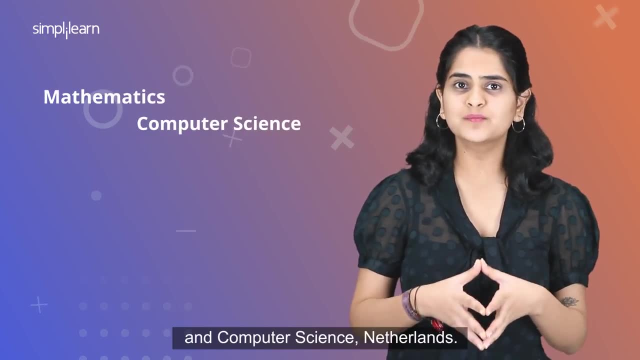 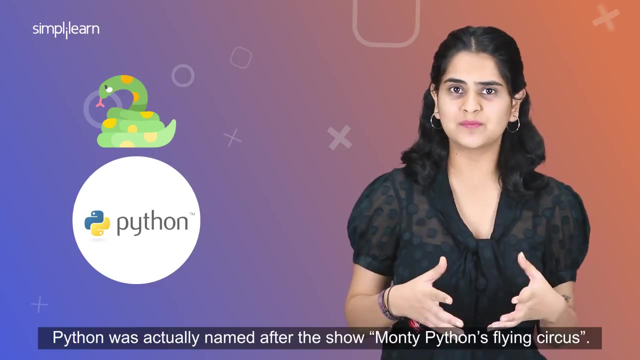 and preferred language. Python is an interpreted high-level general-purpose programming language developed by Guido van Rossum at National Research Institute for Mathematics and Computer Science, Netherlands. In contrast to popular belief that Python was named after this thing, Python was actually named after the show Monty Python's Flying Circus. Guido van Rossum formulated: 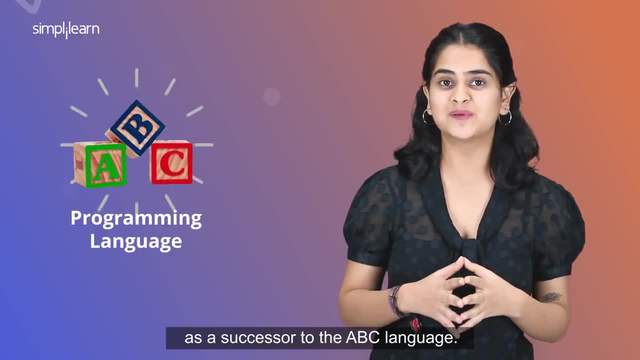 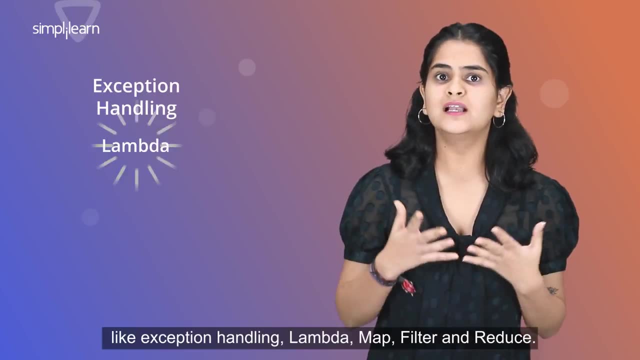 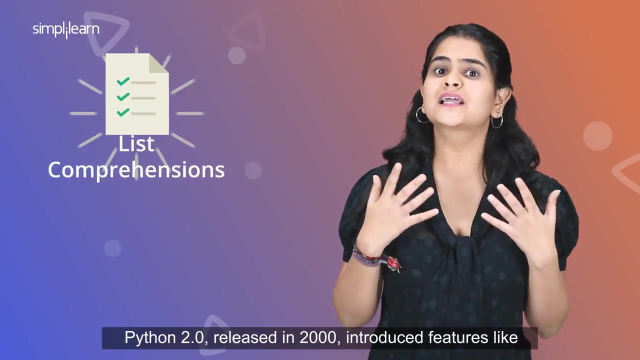 Python in the late 1980s. In 1994, Python version 1.0 was released with features like Exception Handling, Lambda, Map, Filter and Reduce. Python 2.0, released in 2000, introduced features like List Comprehensions. 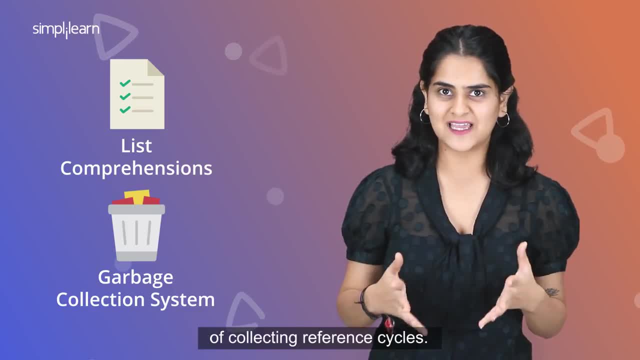 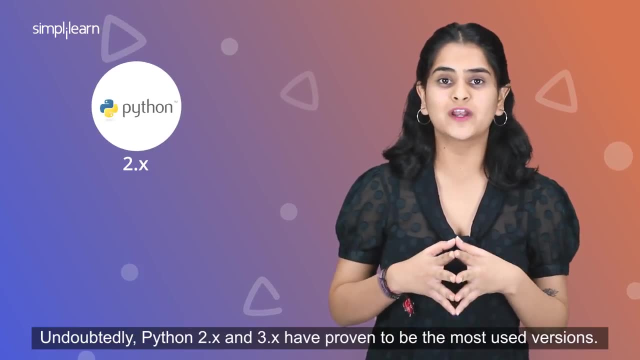 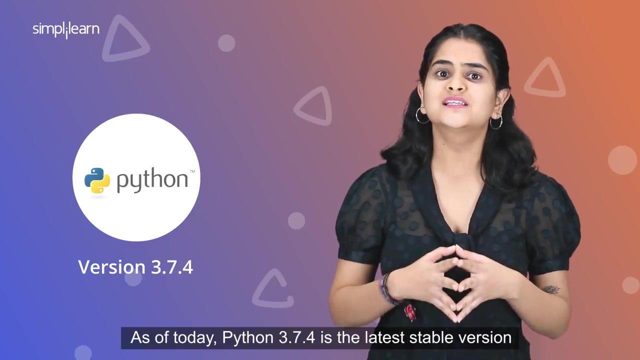 and a garbage collection system capable of collecting reference cycles. Python 3.0 was released on 3 December 2008.. Undoubtedly, Python 2.x and 3.x have proven to be the most used versions As of today. Python 3.7.4 is the latest stable version released in the. 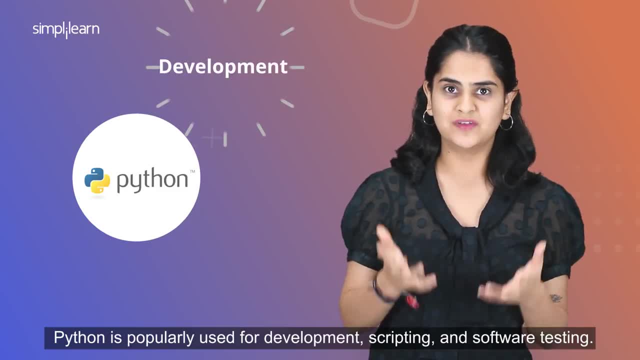 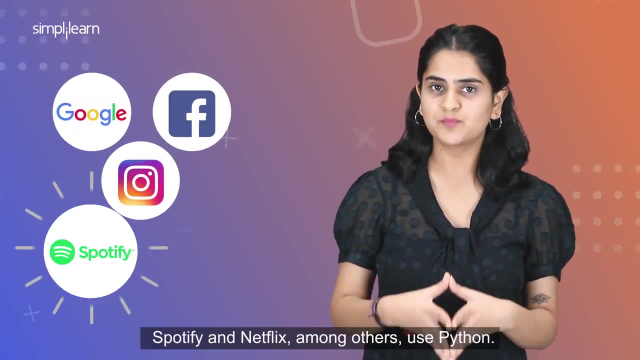 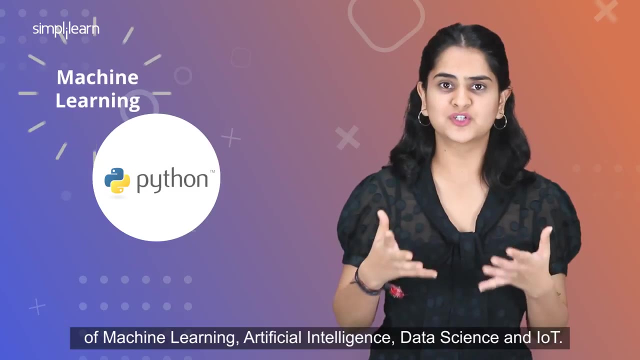 summer of 2019.. Python is popularly used for development, scripting and software testing. Top IT companies like Google, Facebook, Instagram, Spotify and Netflix, among others, use Python. Some major applications of Python can be seen in the fields of machine learning, artificial. 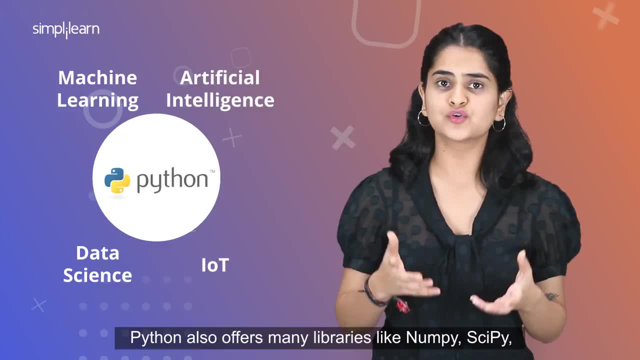 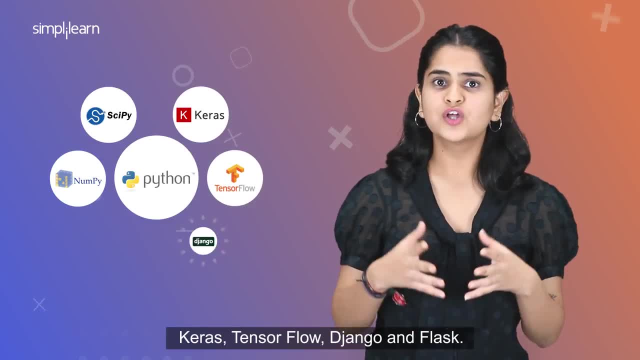 Titan, Python, React, Python Analytics and Photoshop, Python, Mikey Python 2.0. 647 ولسнечт pe ich for Python, Python, Done3D Format and Cl完了 Many libraries like numpy, scipy, keras, tensorflow, django and flask. 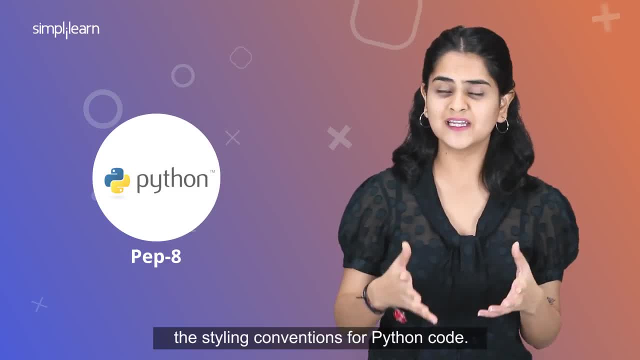 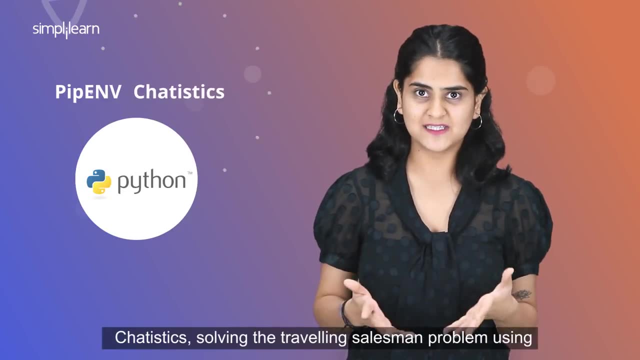 Pep8, Networt 8.0, Numspy Sy версии dan wkszu Jordan. pep 8.0 is the official style guide that defines the styling conventions for python code. A few popular open-source Python projects include pipenv chatistics- solving the traveling. 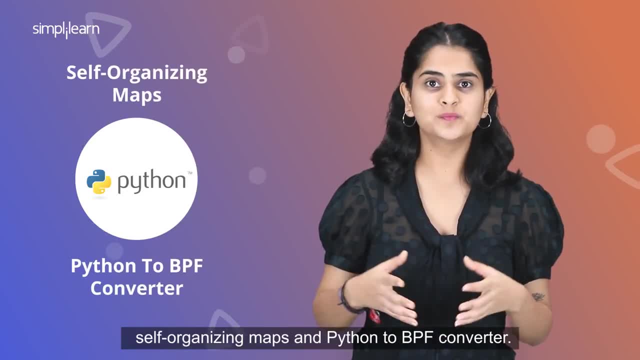 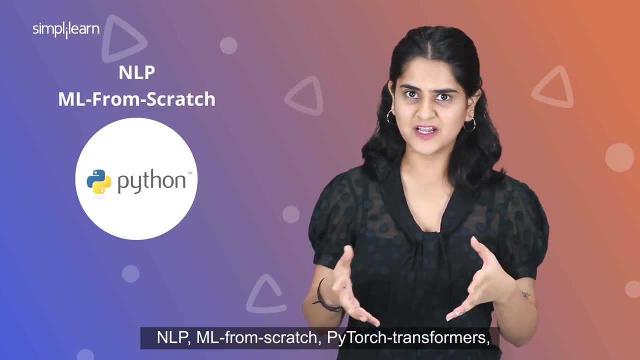 salesman problem using self-organizing maps and python-to-BPF converter. Some of the trending Python repositories on github today include NLP, Msrl, from scratch trainings and smart SOLO spreadsheets, PyTorch transformers, 100 days of ML code, among others. 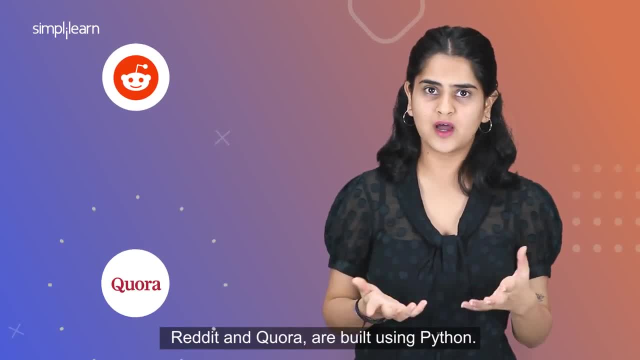 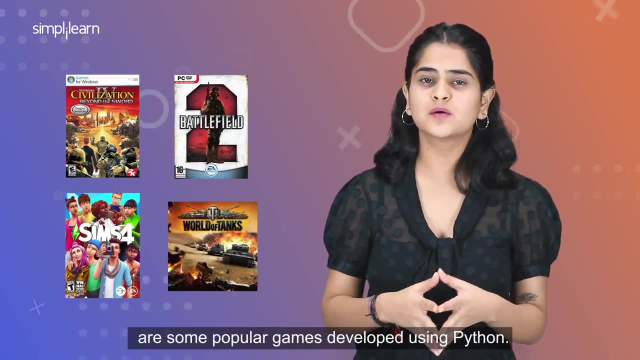 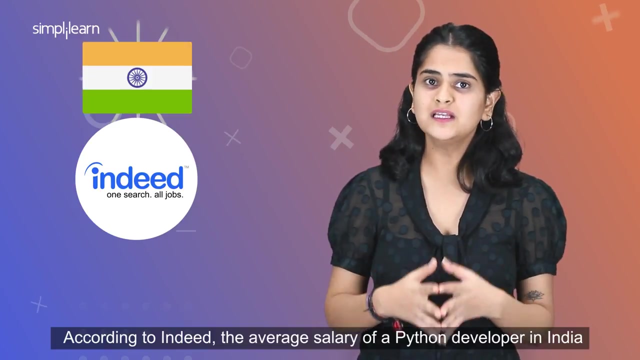 Popular websites on the internet like Reddit and Quora, are built using Python. Civilization IV, Battlefield 2, Sims 4, and World of Tanks are some popular games developed using Python. According to Indeed, the average salary of a Python developer in India is about 5 lakhs per.